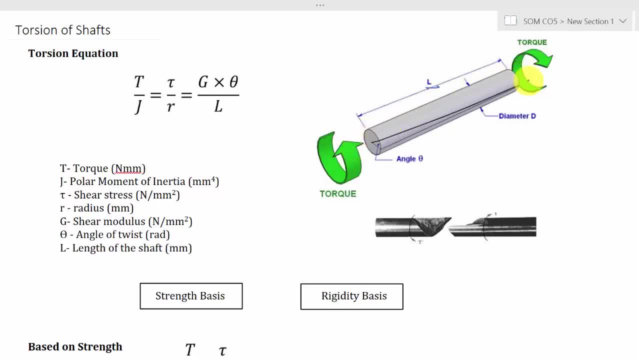 is considered as L. So here a torque is applied. So when the twisting moment is applied, then the shaft will twist to an angle of d eta. So when we are applying a force in this direction, then twisting will occur and the shaft is twisted to an angle of d eta. So this d eta 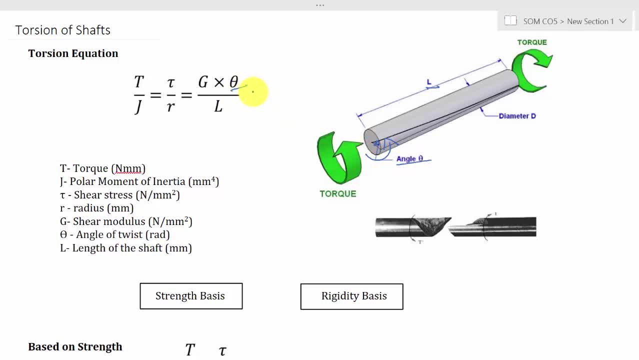 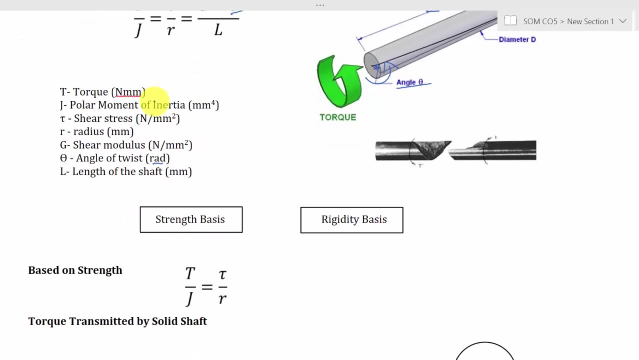 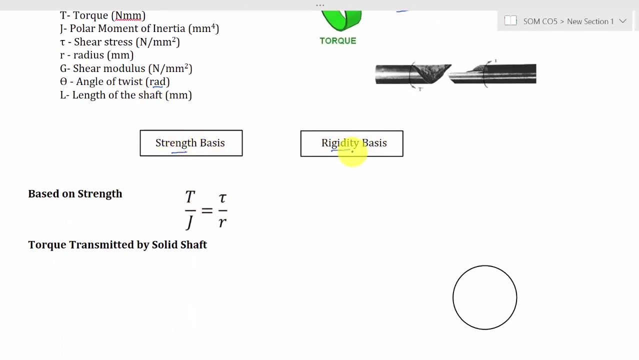 is called as angle of twist. so in the problem when you are substituting the value of theta, you have to substitute in radiant. then L is the length of the shaft. okay, so this is the torque equation. so the design of shafts are based on two things: one is strength and the another one is rigidity. so when the 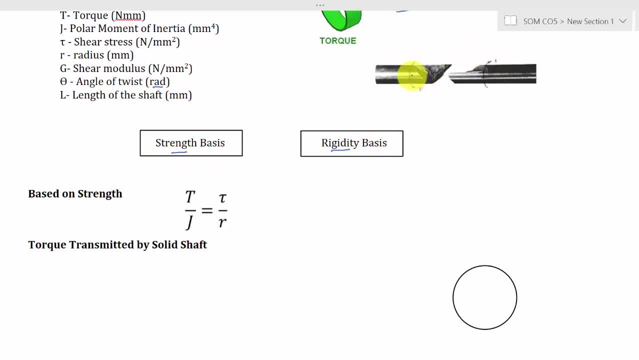 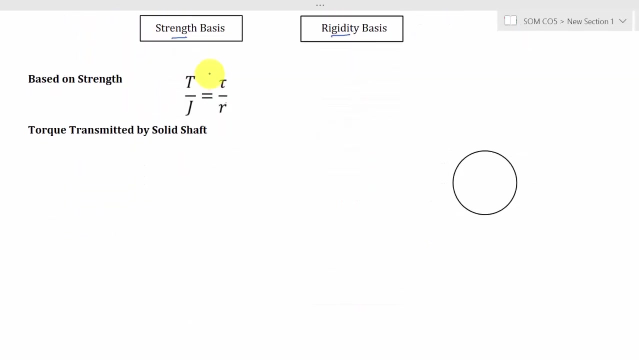 shaft is subjected to torque, then here you can see the image. then the failure will be like this. so this is how the shaft fails. first, by considering the strength. the equation is: T by J is equal to tau by R. so here I have considered only this part, the first two parts. so T by J is equal to tau d tau, by I mean tau. 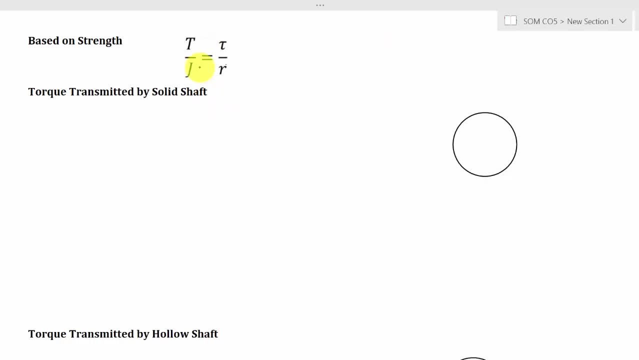 by R. so for a solid shaft, the torque transmitting capacity is: T is reliant, t is equal to- I'm going to write this equation- tau divided by R into J. so here, as I told earlier, J is the polar moment of inertia. and for a circular shaft of solid cross-section with diameter D, we know that. 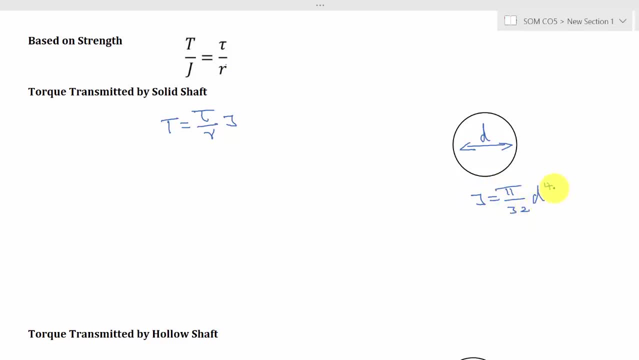 J is equal to pi by 32 D power four. this is the polar moment of inertia equation for a solid circular section going to substitute it. So it is tau into r is the radius. So I am going to write it like this: d divided by 2 into the equation for j is pi by 32 d power 4.. So 2, 32 it is. 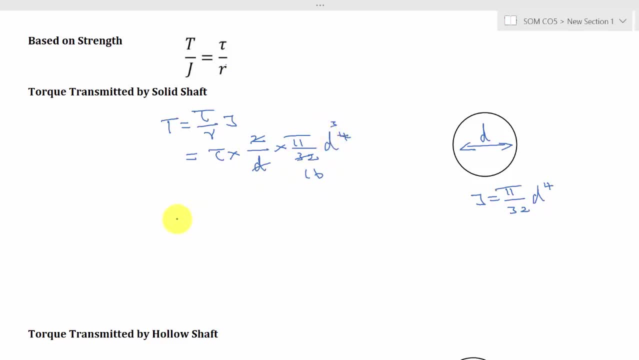 16 and d became d cube. So the final torque equation for a solid shaft is pi by 16 tau into d cube. So this is the equation for the torque transmitting capacity of a solid shaft. So here t is the torque, tau is the shear stress of the shaft material, d is the. 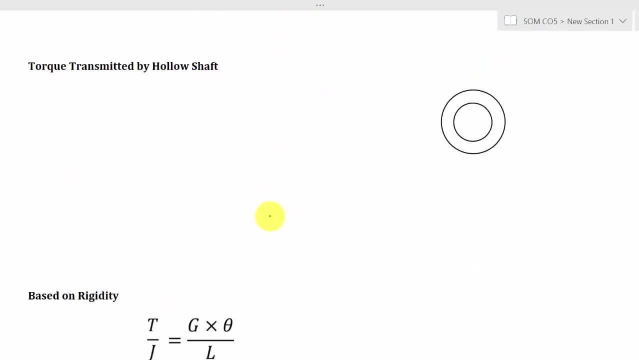 diameter of the shaft. In case of a hollow shaft, then the outer diameter, I am going to consider it as d o and the inner diameter I am going to consider it as d i. So I am going to write the same equation, that is, t is equal to tau by r into j. So t is equal to tau by r into j. and for a hollow 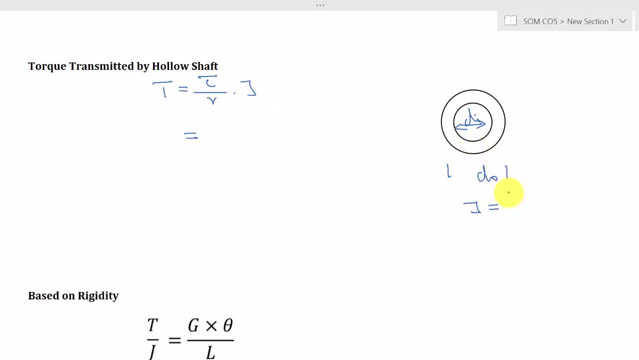 shaft with d o and d i, then the polar moment of inertia is pi by 32. outer diameter, power 4, minus inner diameter, power 4.. So I am going to substitute it. it is tau- into radius is 2 by d- I mean diameter divided. 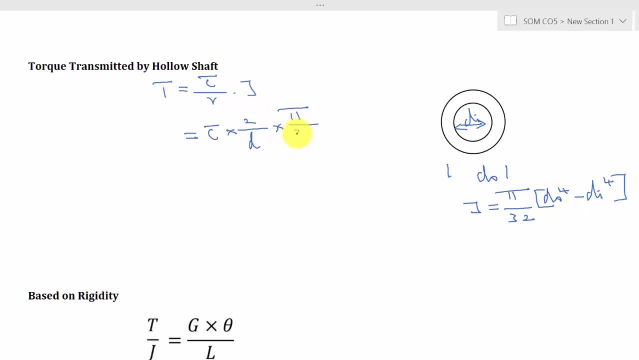 by 2,, then j is pi by 32. outer diameter, power 4, minus inner diameter, power 4.. So here the radius is the outer radius, So here d is the outer diameter. that is very important. Further, if I solve this, then t is equal to 2,, it is 16. So it is pi by 16, tau into. 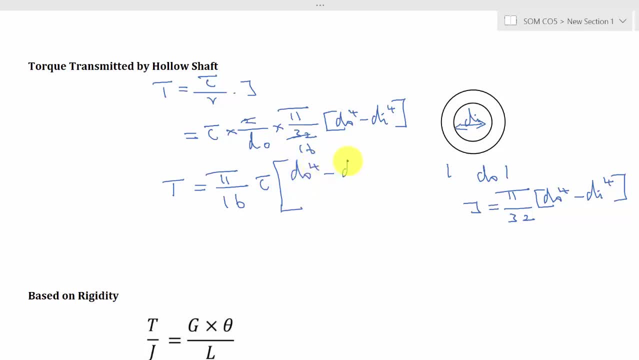 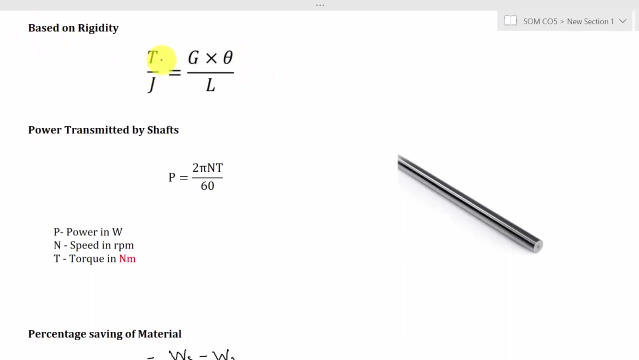 outer diameter, power 4 minus inner diameter. power 4 divided by outer diameter. So this is the equation for torque transmitting capacity of a hollow shaft with d o outer diameter and d i inner diameter. Now the second method is based on rigidity. So when you consider the rigidity, 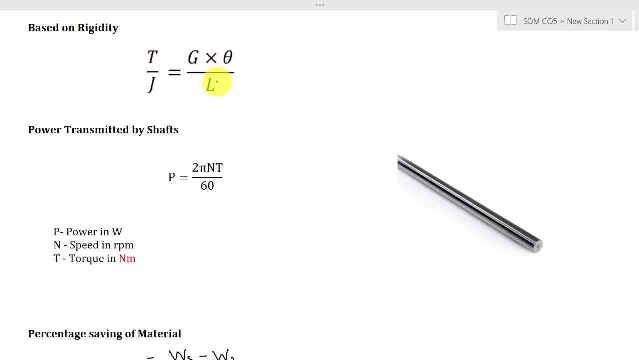 I have considered t by j and g, theta by l, because theta is the angle of twist and g is the rigidity modulus. That is why the design is called as based on rigidity. When you design a shaft based on rigidity, you have to consider the rigidity of the shaft. So you have to consider. 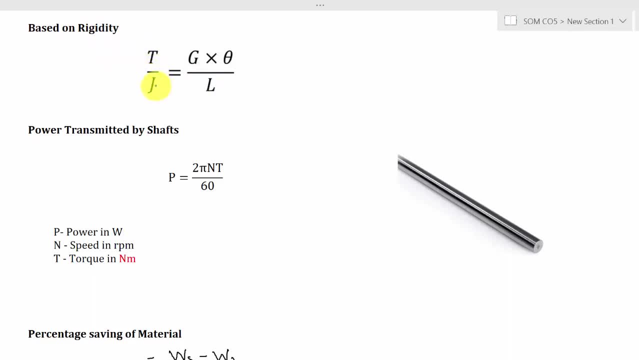 the rigidity of the shaft based on rigidity. So when you design a shaft based on rigidity, you can directly use this equation. You can substitute the value of j, you can substitute the value of g, theta and l and you can calculate the torque transmitting capacity. Now the power. 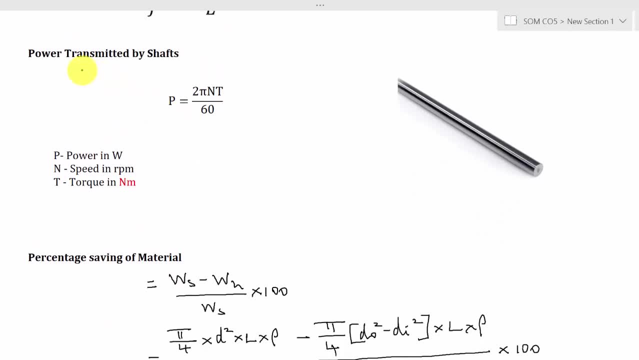 transmitted by the shaft. we know that the equation for calculating the power transmitting capacity of the shaft depends on two things. One is the speed of the shaft and the torque transmitting capacity. So when the shaft is rotating with the torque with some speed, let us say t is in Newton meter and n is in rpm. So that is. 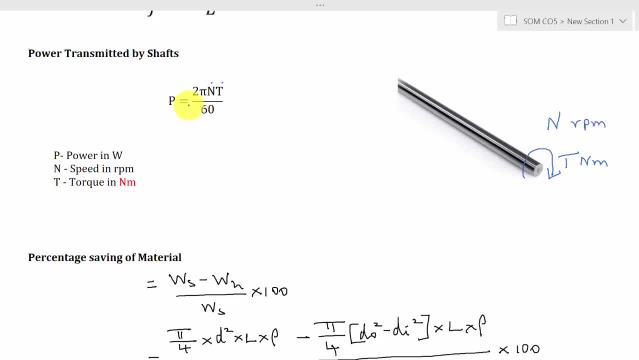 the rotating speed of the shaft. Then p is equal to 2 pi n t divided by 60. So remember that you have to substitute the torque in Newton meter in this equation. You should not substitute the torque value in Newton mm. So that is very important When you substitute the torque in the power. 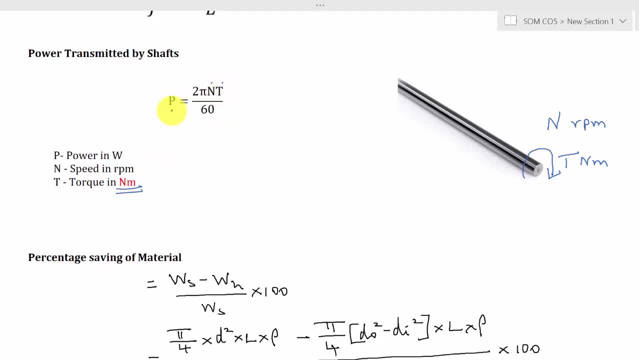 equation. you have to substitute it in Newton meter, So that is very important. When you substitute the torque in Newton meter, you shall get the power value in watt, So that is very important. Keep this in your mind while solving the problems. 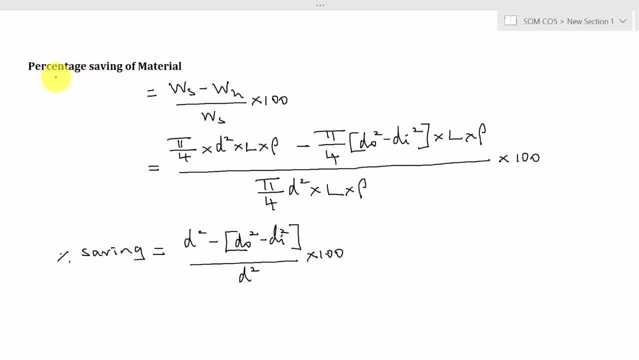 Then the next one is: in some of the problems they may ask you to calculate the percentage saving of material. So here the percentage saving of material equation is weight of the solid shaft minus weight of the hollow shaft, divided by weight of the solid shaft into 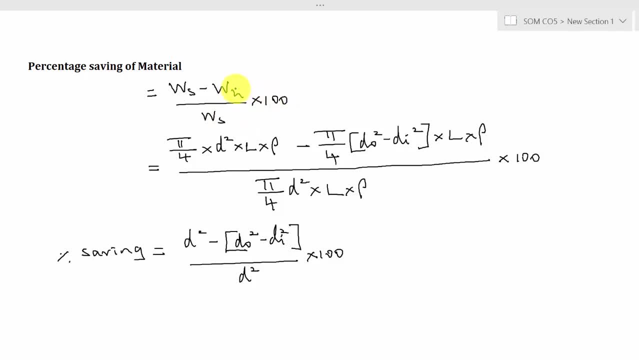 100.. 0.614원, Because the hollow shafts will transmit more torque, but the weight of the hollow shafts will be very low. That is why we are calculating the percentage saving of the material. So here Ws is the weight of the solid shaft, Wh is the weight of the hollow shaft, and we 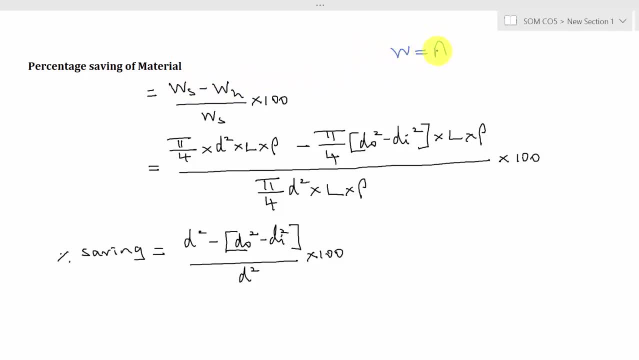 know that to calculate weight the equation is area into length, into density. So actually this area into length will give you the volume and by multiplying the density with the volume we will get the weight. And for circular cross section the area is pi by 4 d square L into rho.